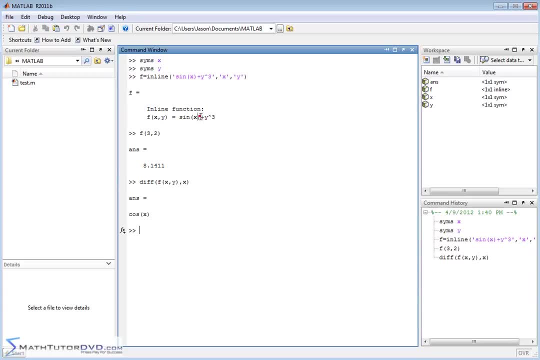 then this is the answer I get. Now, if I look at my original function up here, if I take my derivative with respect to x, then this y cubed is just a number, it's just a constant, so it drops away when I take the derivative. 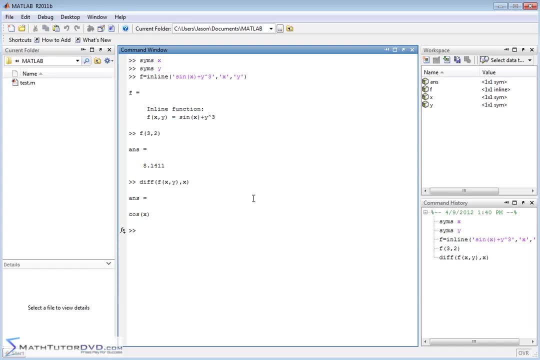 And the derivative of sine is cosine, so that's calculated correctly. If I pull up the last command and just replace this with a y, then I'm going to do the other guy. I'm going to pretend that x is constant, so it's going to drop off. 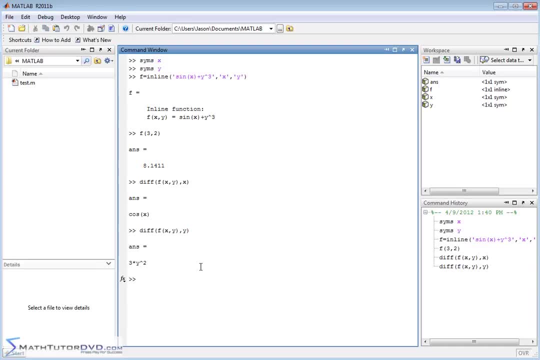 and the derivative of y cubed is simply 3y squared. So in a large picture, in a big picture, that is how you handle multivariable functions in calculus. In fact, we could create a third symbol variable and call it z right. 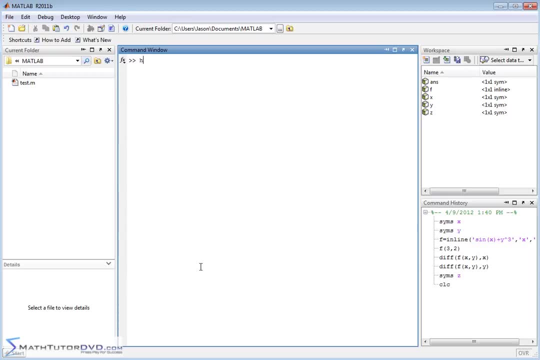 So now we have three symbol variables and I could create another function and h of, or I should say h is equal to inline and I could just create anything I want. I could say: you know, x to the 10th minus y squared plus log of z. 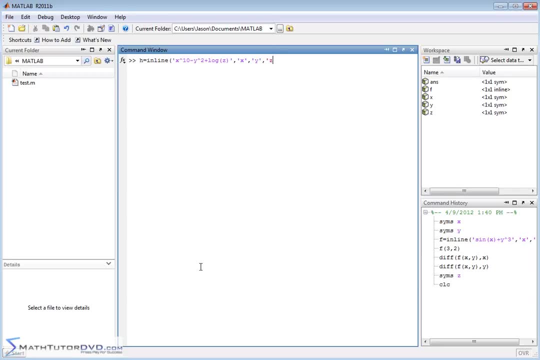 And x, y and z are the independent variables. So I've created a function of x, y and z and I'm telling the MATLAB that the independent variables are in fact x, y and z. so my inline function is written. 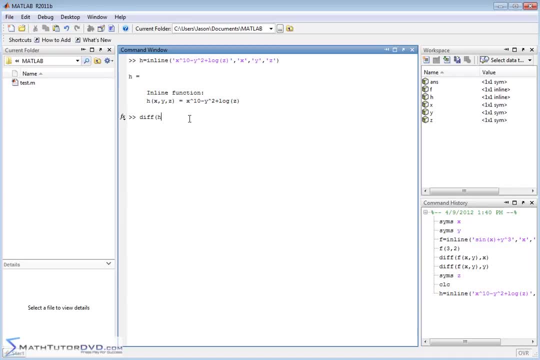 just as it is there, right. And then I can take the derivative of h, x, y, z and I have to pick a variable to take the derivative with respect to. If I pick x, MATLAB's going to hold everything else constant. 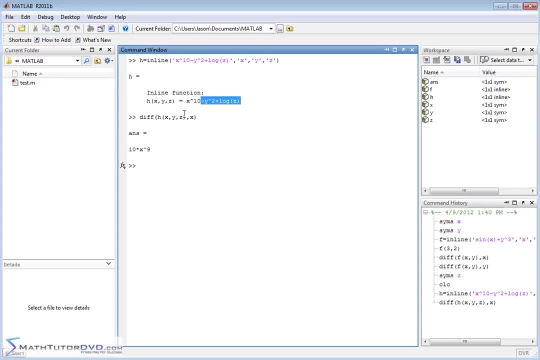 So all the stuff here in this case would be constant. So the answer I get is 10x to the 9th. If I pull the command back up and I take the derivative with respect to y, then this is held as a constant, so it drops off. 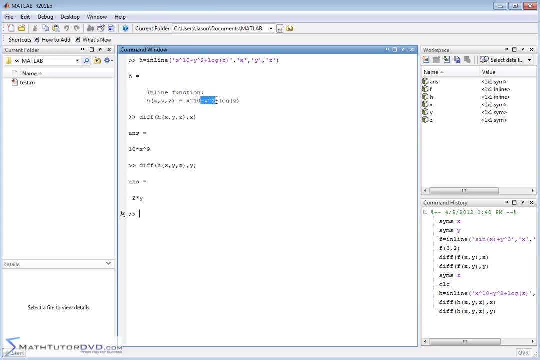 This is held as a constant, it drops off and the answer I get for the derivative is negative: 2y. And finally, if I calculate the derivative with respect to z, the partial derivative with respect to z, I'm going to get this 1 over z. 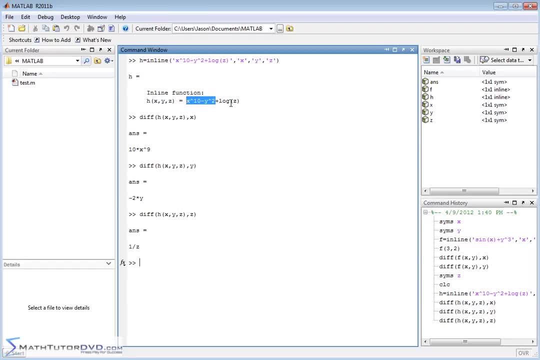 because all of this stuff is a constant and it drops away and the derivative of a logarithm is just 1 over the variable. So partial derivatives really are handled exactly in the same way that regular derivatives are handled. There's no separate function for it. 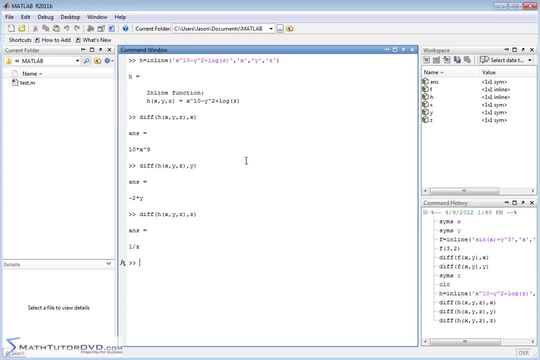 It's just that you have a multivariable function in here to begin with. All right, so now what I want to do is go and show you how to calculate a derivative of a function of more than one variable and evaluate that derivative at a point. 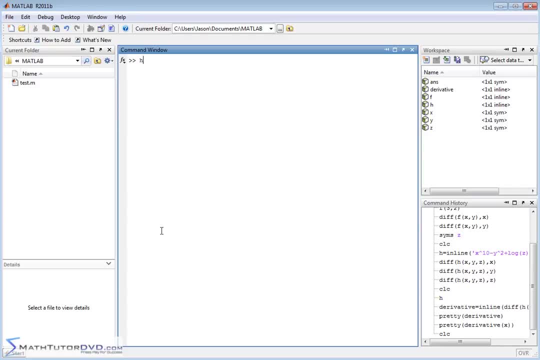 So what we're going to have is: let's go ahead and calculate or create a new function. We'll call it h and we'll say that it's equal to. let's make it a function of two variables, to make it a little bit easier to handle. 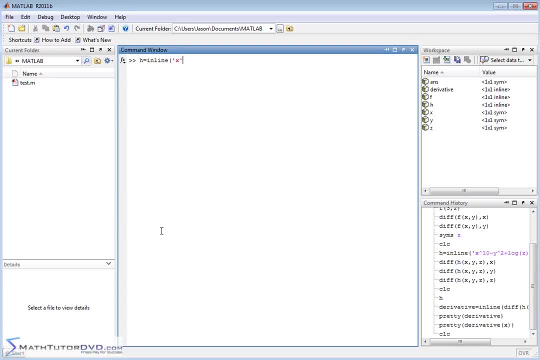 So we'll have x, let's say x cubed. let's just say y times x cubed. Let's do it like that, Actually, just to make it a little easier to read. we'll have x times y cubed. 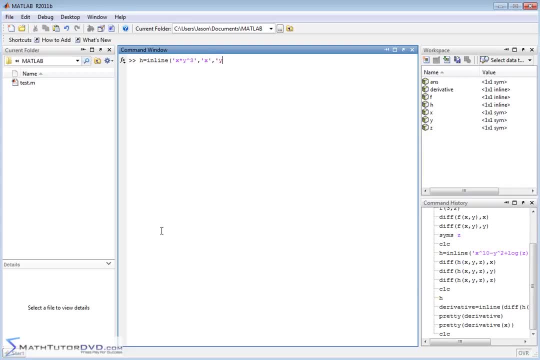 So that'll be our function, And of course it's a function of x and a function of y. So we create the function and that makes sense exactly the way it's written there. Now we want to calculate the derivative. Now we know we can pass this to the diff operator. 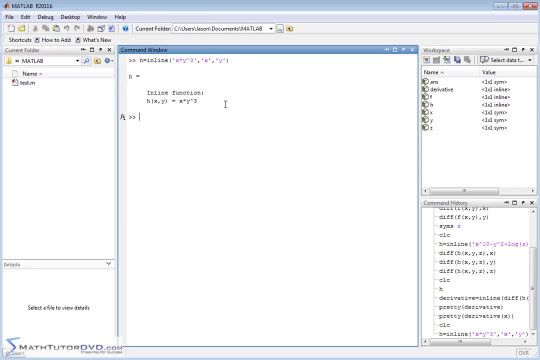 the diff function and get the value back. But we want to define a function so that when we get our answer we can plug numbers into it, right? So let's go ahead and calculate. let's calculate the derivative, And to do this we'll have to see. 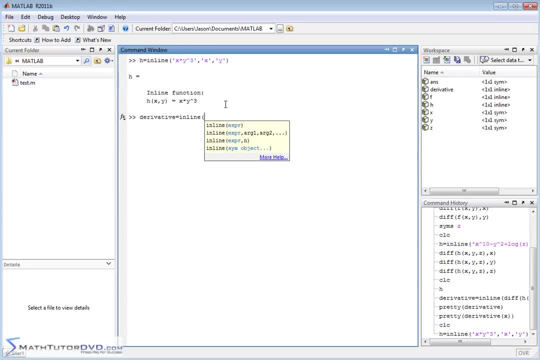 if we can set it equal to an inline function which just tells MATLAB: create a function for me. What function am I creating? Well, you're calculating the derivative. You're calculating the derivative of h, of x, comma, y, and you're calculating the derivative. 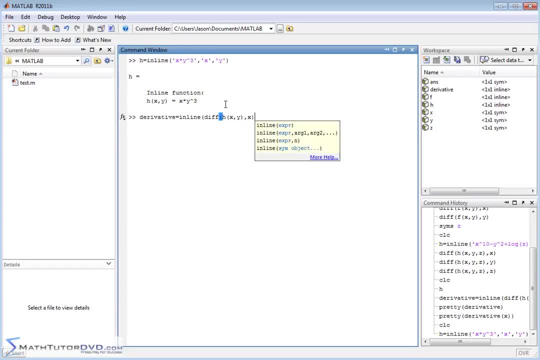 let's say, in this case, with respect to x, All right, whatever you can just pick, your pick, whatever you're trying to do. But let's just say we're taking our h of two variables, our function of two variables. 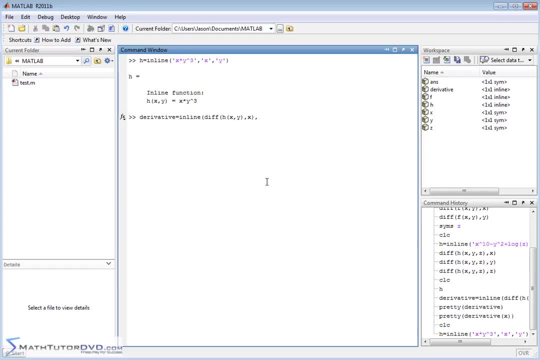 we're calculating the partial derivative with respect to x and we put a comma here because we have to. don't forget: this is an inline function, It's creating a function. The final function we get is going to be a function of x. 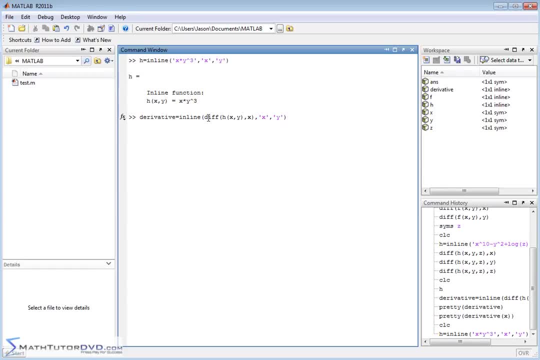 and a function of y. So make sure you understand what we're doing. We're taking the derivative of this function with respect to x. That's what. that's the function we're creating. inside this inline parentheses, The result of it is going to, in general: 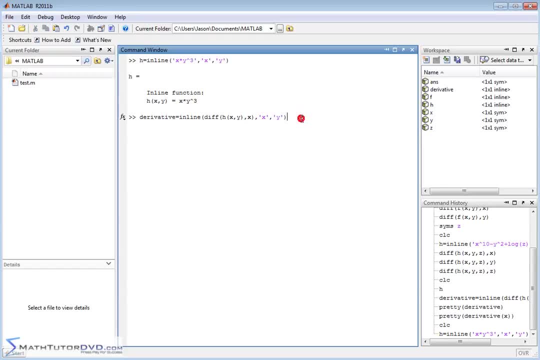 be a function of x and y And we're setting this equal to the derivative label that we have. So we hit enter and it creates our. it creates our function, right? So in this case it's y cubed, because this is a fairly simple function. 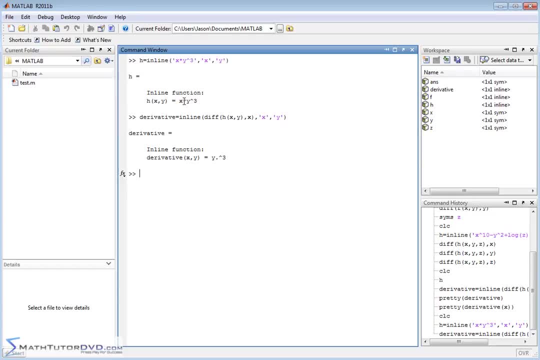 x times y cubed. When you take the derivative with respect to x, then you basically hold y constant right. So you hold y constant and this is the value that you're going to get. So you can take derivative one comma one. 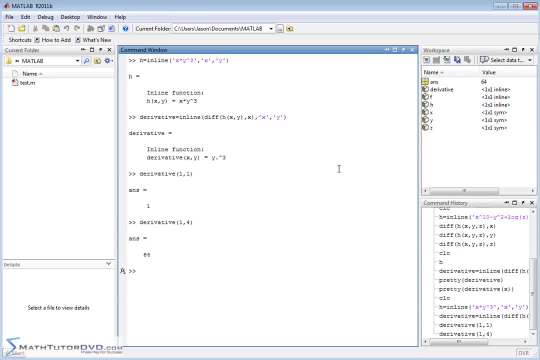 and it'll calculate a value back. You know, one comma four, it'll calculate a value back Now if we go back up a little bit and change our original function to something a little more complicated. So instead of of of something like this: 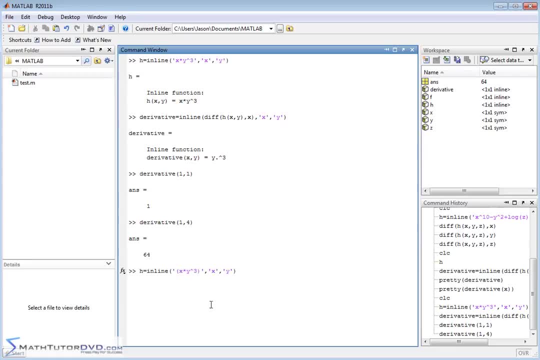 let's do it like this: We'll put parentheses on the top and then we'll put a division bar and we'll do x plus y. So this is a much more complicated function. So what we're doing now is we're redefining h. 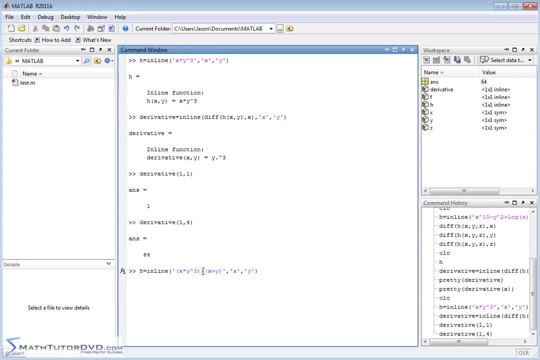 to be x times y, cubed on the top over x plus y on the bottom. So this is now a new function. You can see it right here, And we're going to go up a few other commands and let's assign. 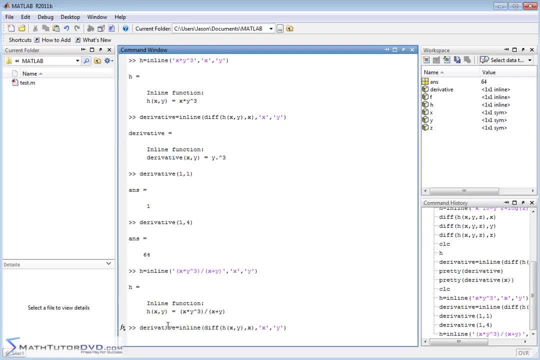 let's assign the label derivative. to calculate the derivative, set it equal to a new function that we're calling derivative. We're again taking the derivative of our h function with respect to x and our new function is going to, in general, be a function of x and y. 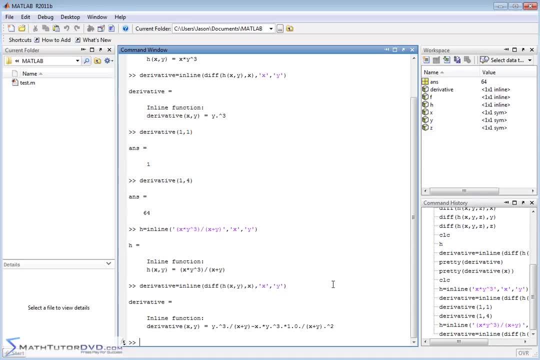 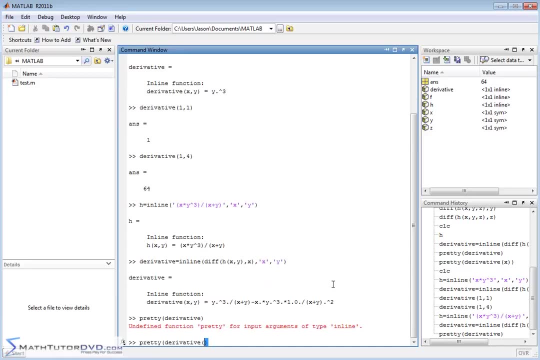 So we hit enter and here's our nice ugly looking derivative. We can fix that by taking derivative and basically sticking it in the pretty function, And we have to specify the arguments x, comma, y. all right, And so here's our derivative right. 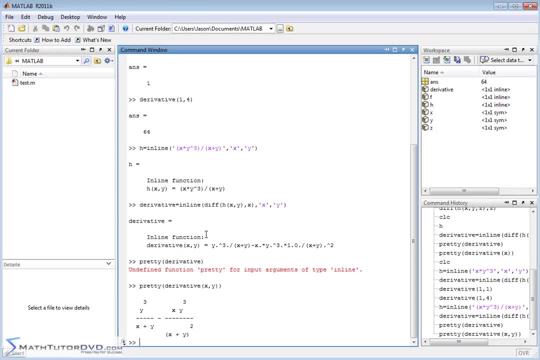 So y cubed over x plus y minus all this stuff. So basically, what we're doing is we're taking the derivative with respect to x, we're sticking it in the inline argument to create a new function, which is always, in general, going to be. 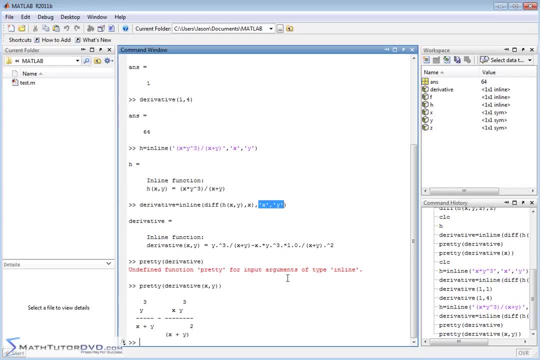 a function of x and y. This is just like regular old calculus. When you take a two, a function of two variables, you take a partial derivative. the function you get back is in general going to be still a function of two variables. 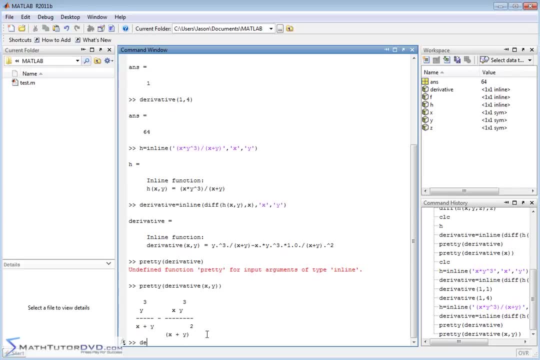 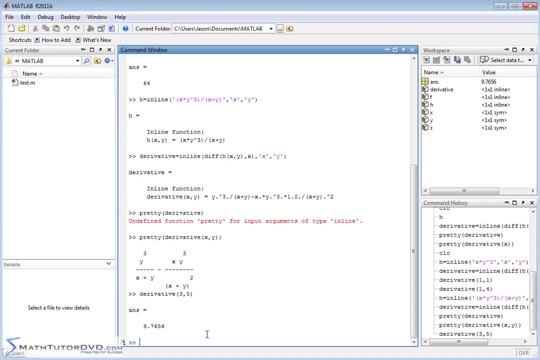 And that's what we have here. And when you do it this way, you can take that derivative and put whatever you want in there And it'll calculate a single value back. So you can plot this, You can perform additional calculations or functions on this new function.